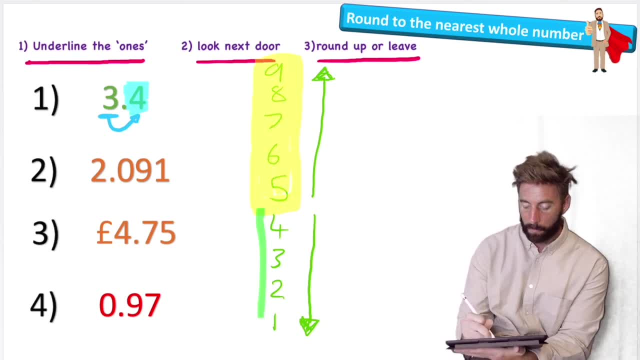 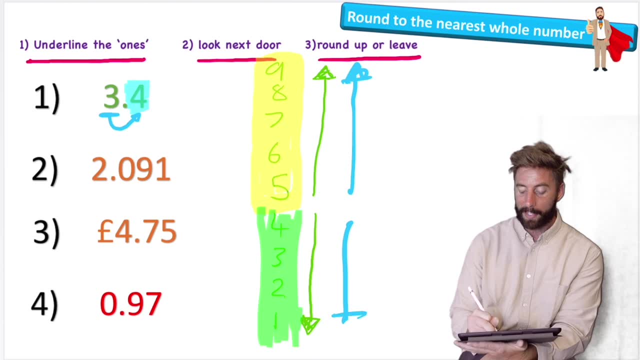 So nine, eight, seven, six, five, we round up Four, three, two, one. we round down Five or more, let it soar. Four or less, let it rest. Okay, so, using this knowledge, let's see what we're going to do to this four, that's next to our three. 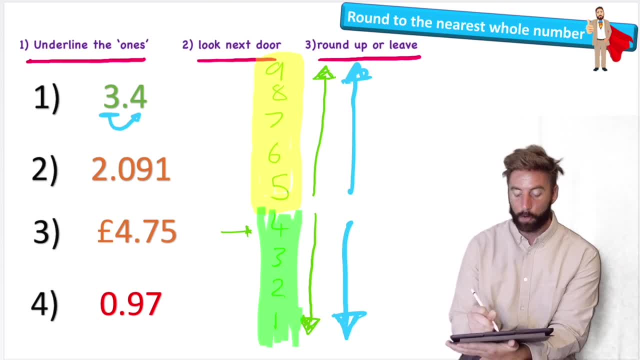 Well, the four is here, And remember one, two, three, four, Four or less. let it rest. So we would end up leaving the three as a three, We would not round it up to a four, So the number would be three. 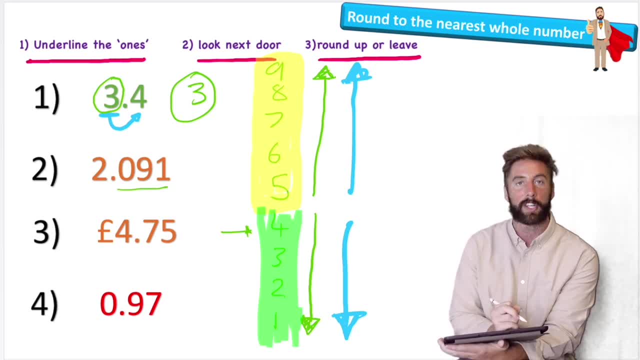 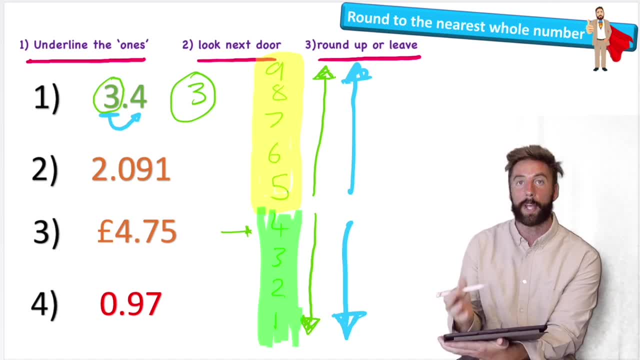 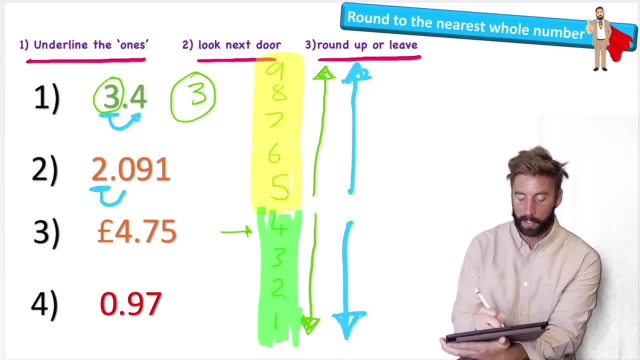 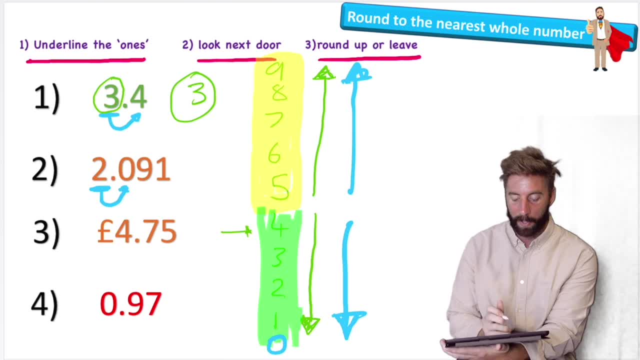 Okay, number two looks a little bit more difficult because there's extra digits after our definition. Okay, number three looks a little bit more difficult because there's extra digits after our definition. Okay, number two looks a little bit more difficult because there's extra digits after our definition. 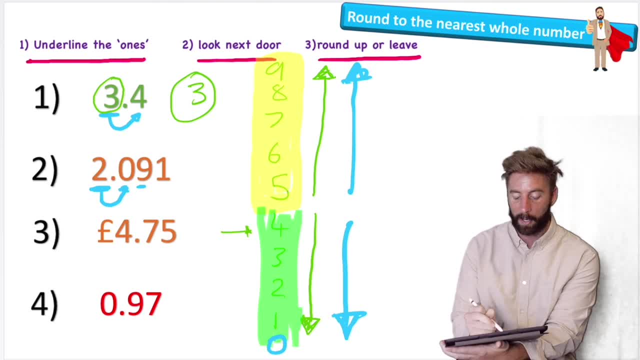 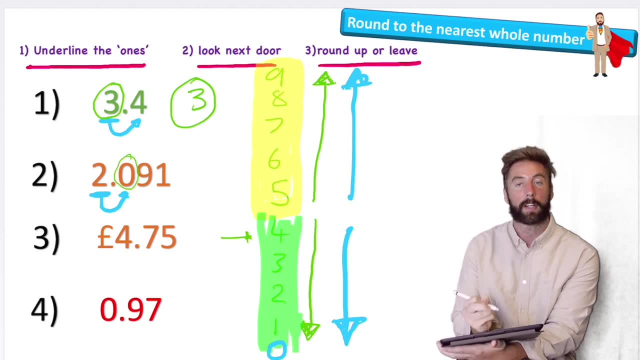 That doesn't influence us, because we only look next door to the one digit, next door to the right. So, looking at my zero, what am I going to do? That's right, I'm going to let it rest. so 2.091 becomes just the number 2.. 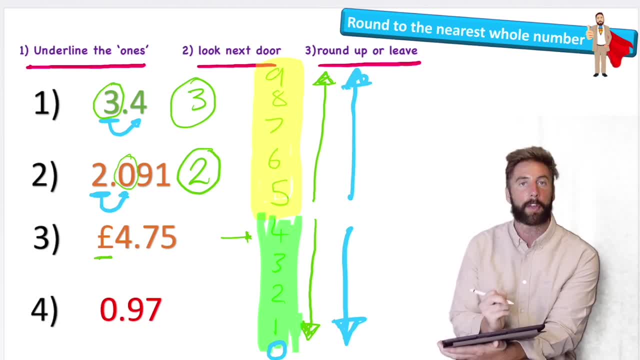 Okay, number 3, and I've used one here with the pound sign because this is a very common question that you're going to get. How do we round these pence up to the nearest pound? So this says £4.75, and a question typical in a SAT exam, for example, would say: round this to the nearest pound. 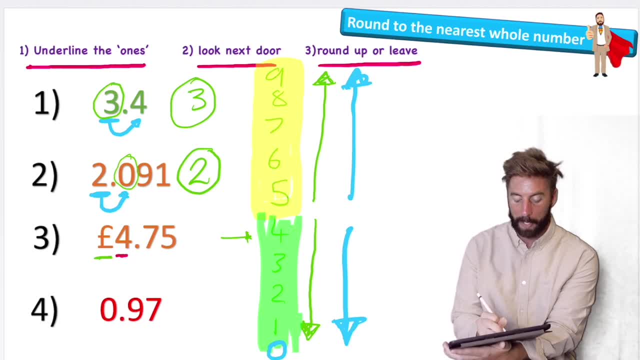 So same thing. our nearest pound would be here in our ones column, And all I'm going to do is look next door and we have a 7. Where is 7 on our list? It's here. And remember the phrase: 5 or more, let it soar. 4 or less, let it rest. 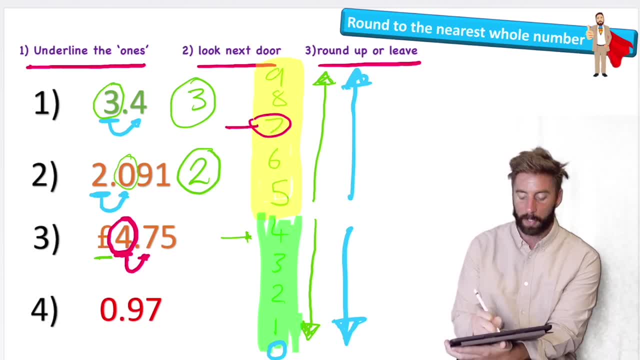 We're going to soar this 4 up here Up to a 5.. So my answer to question 3 would be £5.. Okay, question 4, 0.97.. Again, looks a bit more tricky because we have the zero here. might confuse us.